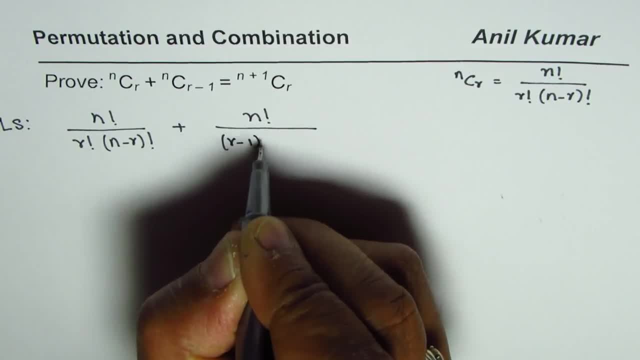 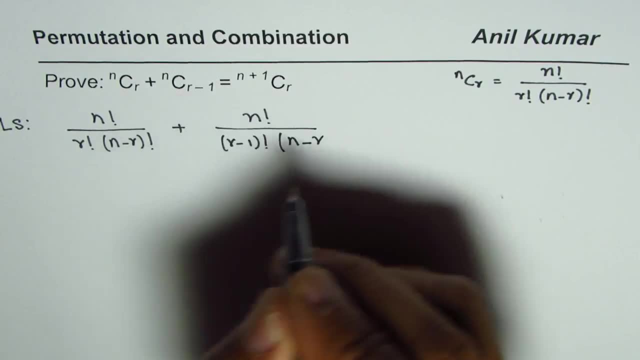 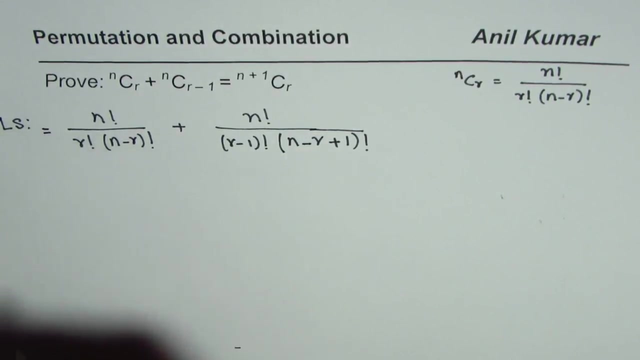 divided by r, factorial, r minus 1 factorial times n minus r and minus of minus 1 becomes plus 1, correct factorial. So that is the left side for us. So this is equal to left side. Now we have to add them. 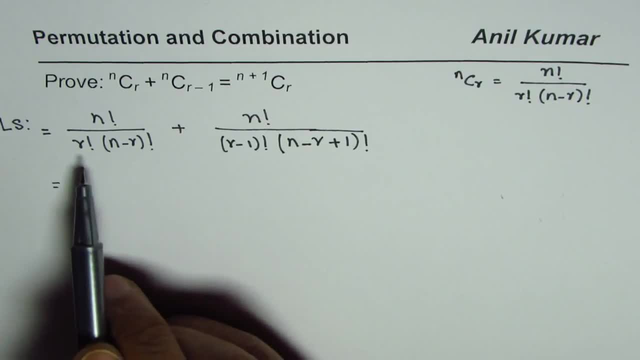 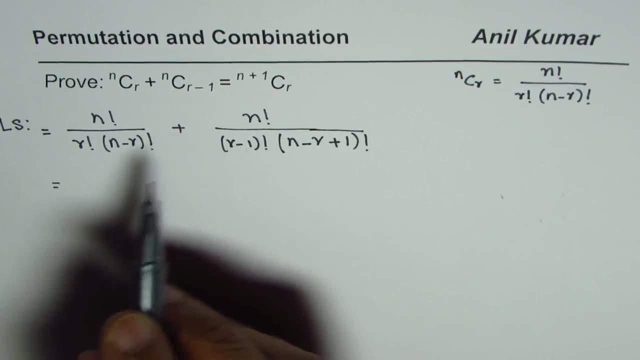 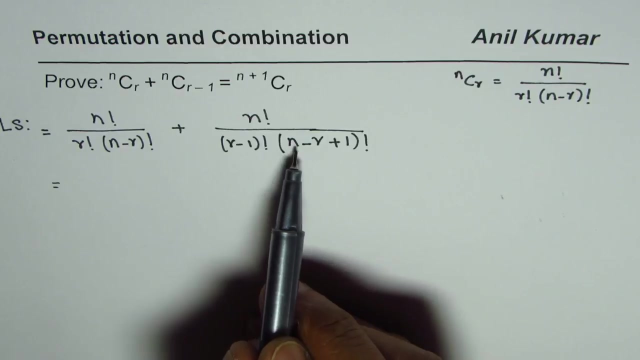 To add, we should have common denominator. Now, here we have r factorial. In this case it is r minus 1 factorial. We need to multiply this by r. right On the left side we have n minus r factorial. Here we have n plus 1 minus r factorial, Do you? 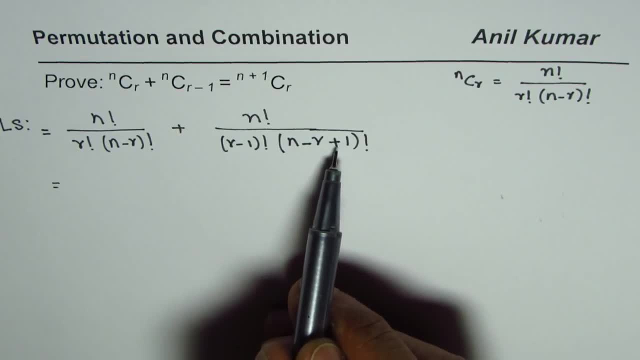 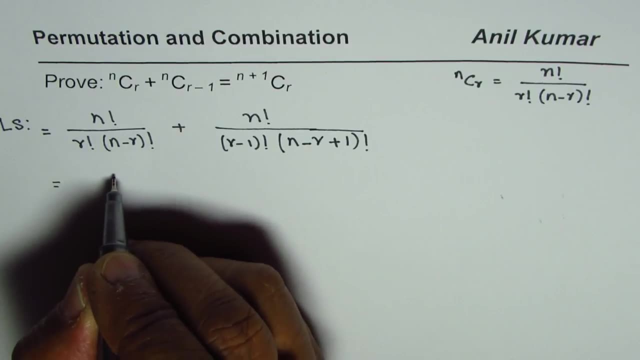 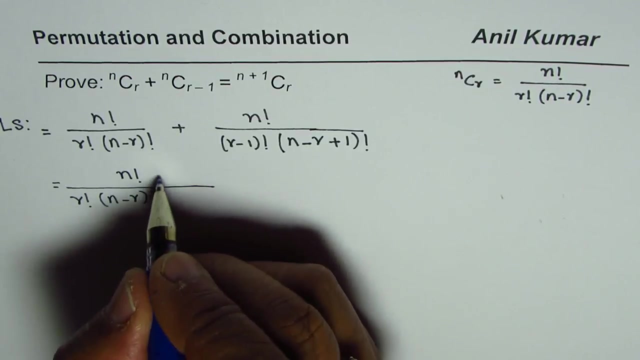 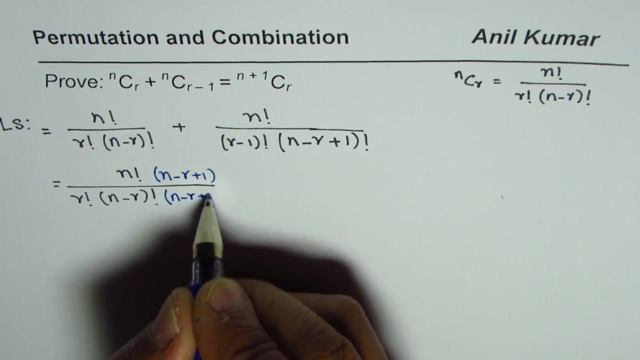 see that. So that means we have to multiply this by n minus r plus 1.. So let us do that. So what we are going to do now is we have n factorial divided by r factorial times, n minus r factorial. We multiply this by n minus r plus 1 in the numerator and n minus r plus 1 in the denominator. 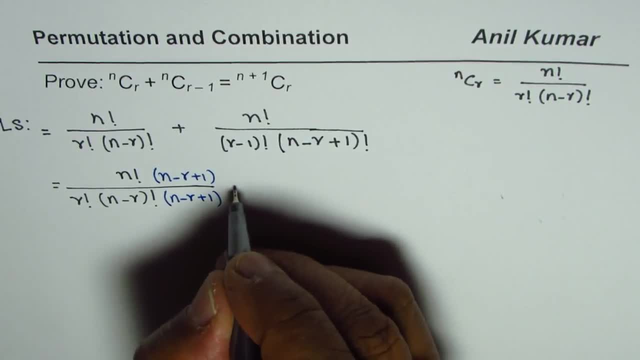 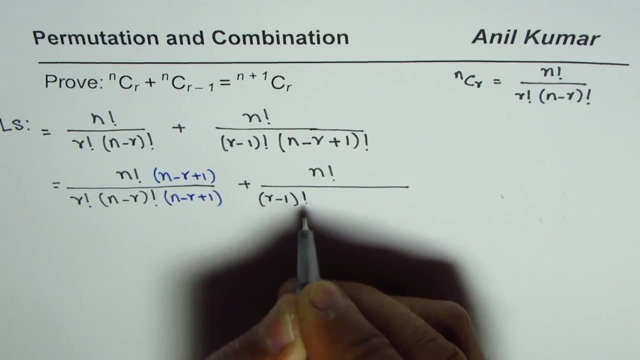 correct. Now what we are going to do in this case is we are going to multiply this by r, by n minus r, factorial in the denominator For the other term, which is n. factorial by r minus 1. factorial times n minus r plus 1. 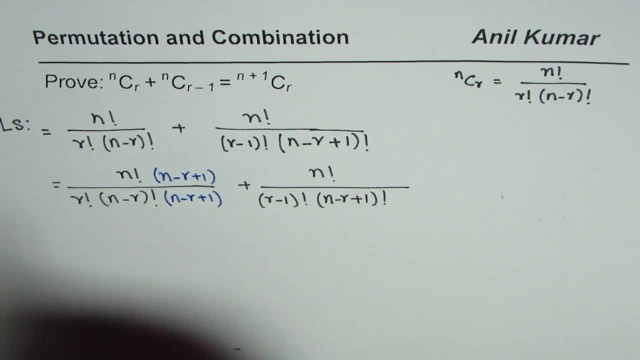 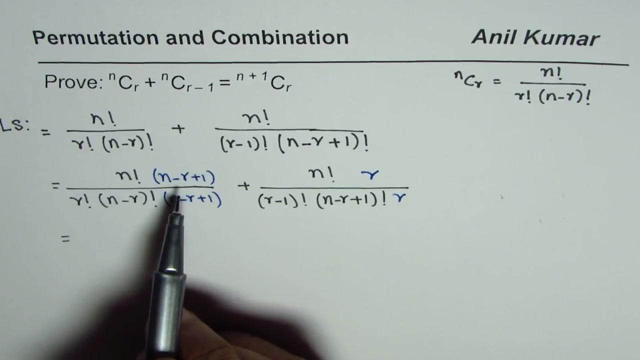 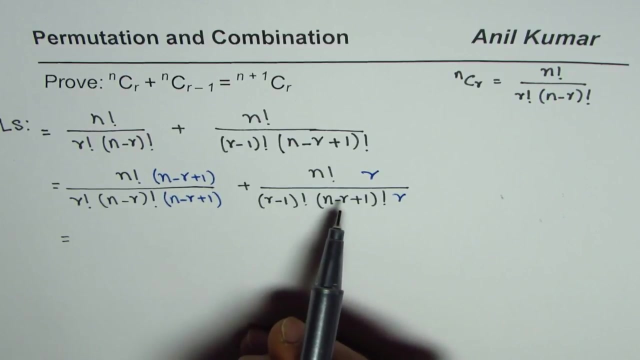 factorial. we are going to multiply this by r, correct? So we multiply this by r in the numerator and r in the denominator. Now, by doing so, we can actually write the terms in the numerator and the denominator with common denominator. do you see that? So that is the whole idea. 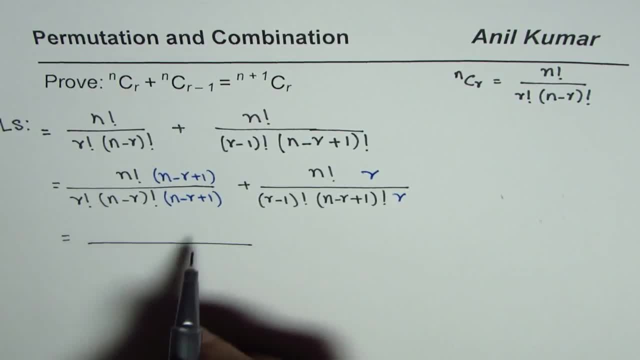 So the denominator could now be written as r factorial. this is also r factorial right, So we have r factorial and n minus r plus 1 factorial right, So which you could write this as n plus 1 minus r factorial right, So that times this. here also we have the same denominator. 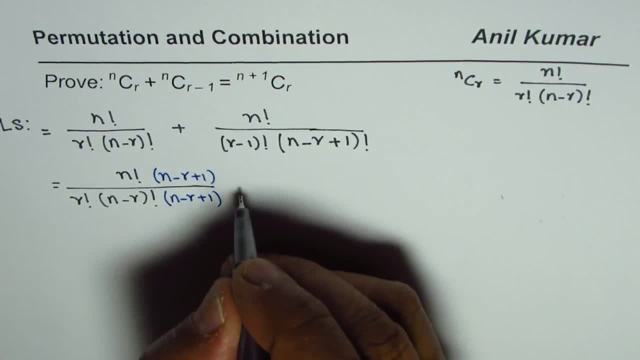 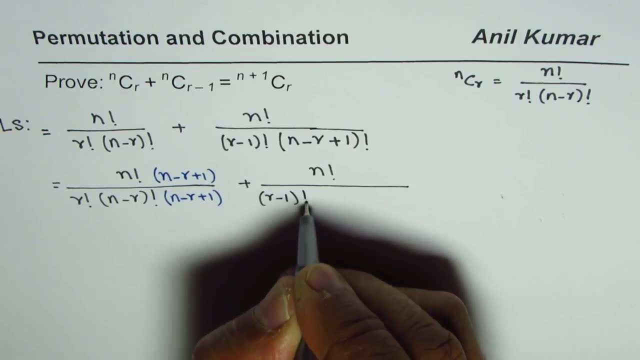 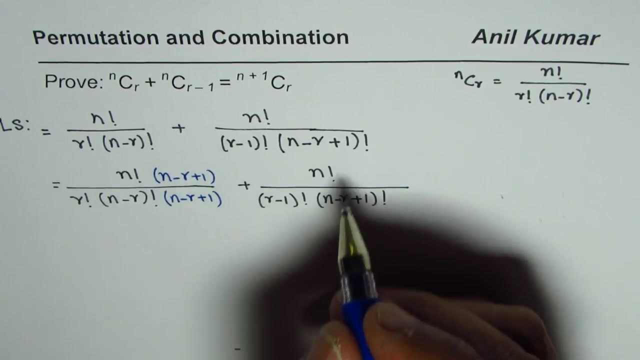 1 in the denominator. correct For the other term, which is n factorial, by r minus 1 factorial times n minus r plus 1 factorial. we are going to multiply this by r, correct? So we will multiply this by r in the numerator. So we are going to multiply this by r in the numerator. 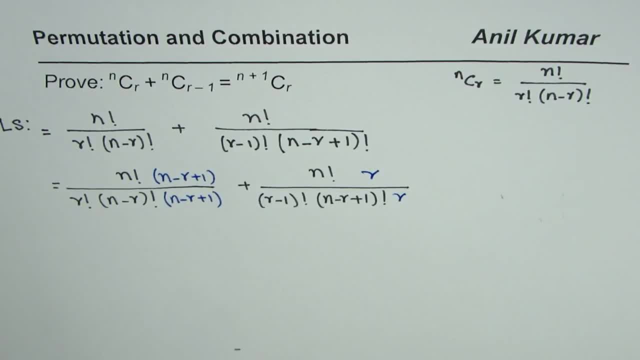 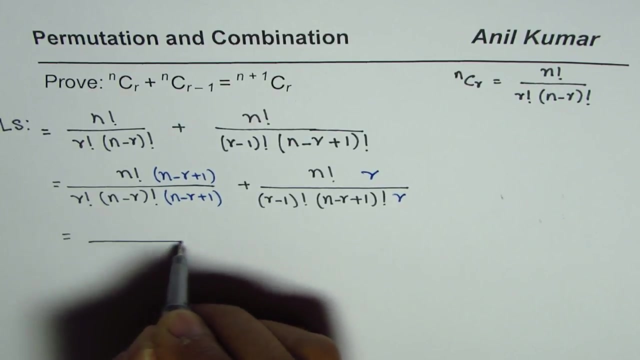 and r in the denominator. Now, by doing so, we can actually write the terms in the numerator and the denominator with common denominator. Do you see that? So that is the whole idea. So the denominator could now be written as r factorial. this is also r factorial, right. So 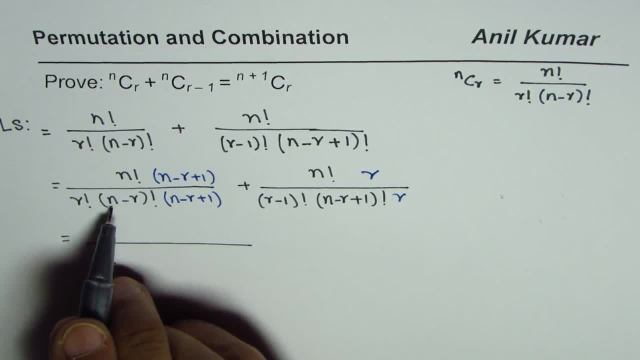 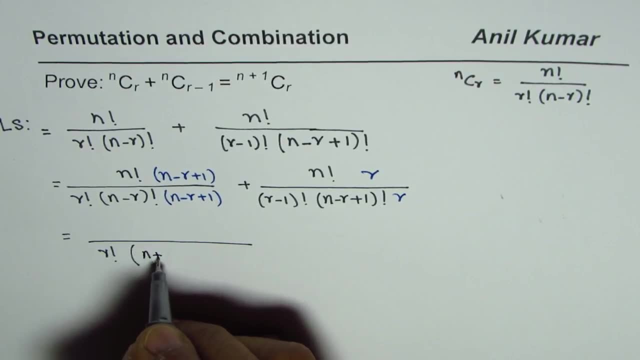 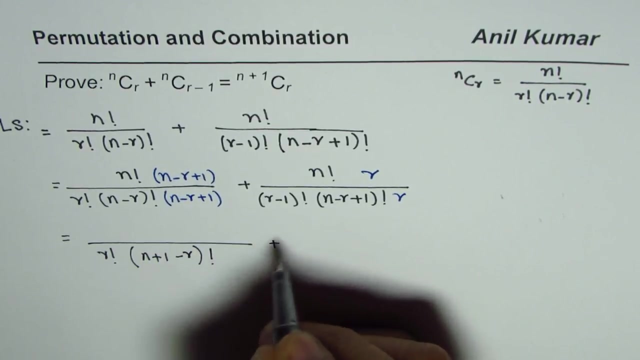 we have r factorial and n minus r plus 1 factorial right, which you could write this as n plus 1 minus r factorial right, So that times this- Here also we have the same denominator, Which is r times r minus 1 factorial is same as r factorial, and this one could be rearranged and: 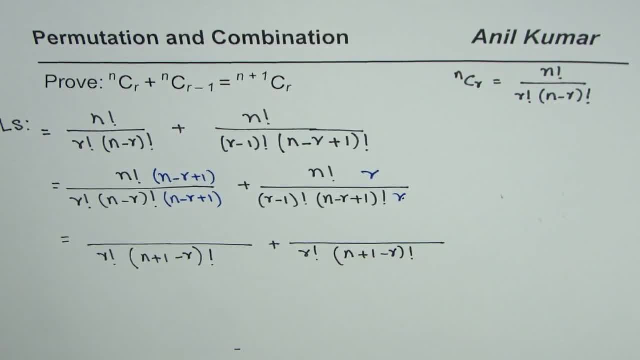 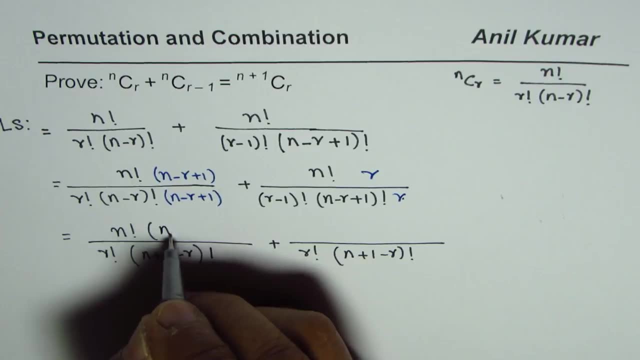 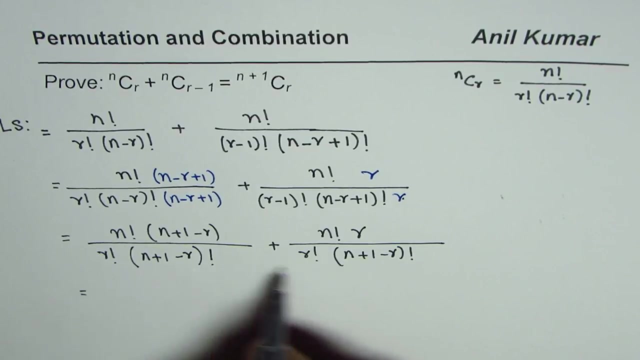 written as n plus 1 minus r factorial, And the numerators for us are n factorial times n plus 1 minus r, and this is n factorial times r. Now, since the denominators are same, we can take them. So what we have here is 1 over r factorial times n plus 1 minus r factorial, and in the 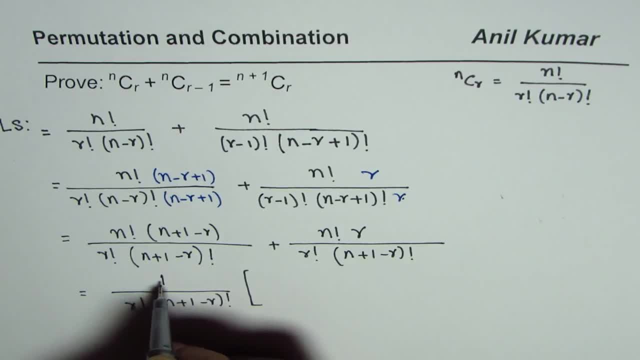 numerator. let us add them. I should actually take n factorial also common, right? So we have n factorial also common. We have the terms n plus 1 minus r, and here we have plus r. Now what you will get is n factorial times n minus 1 minus r. factorial into n plus 1. 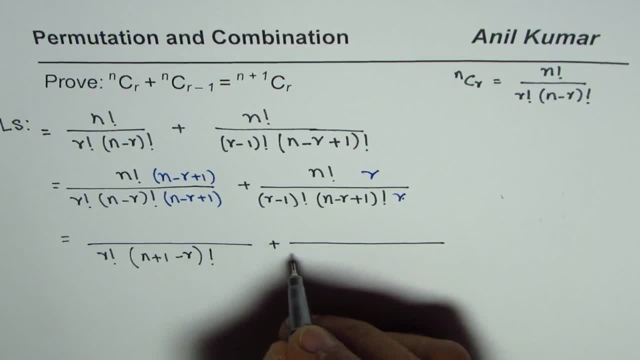 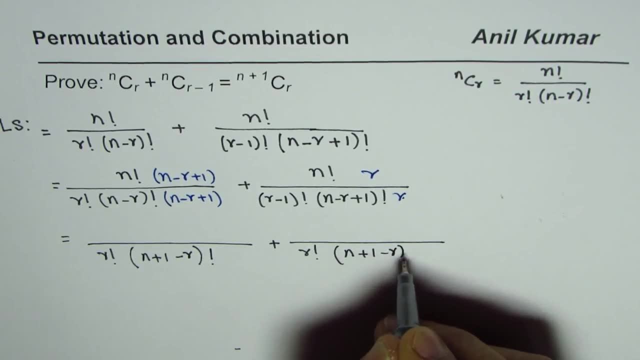 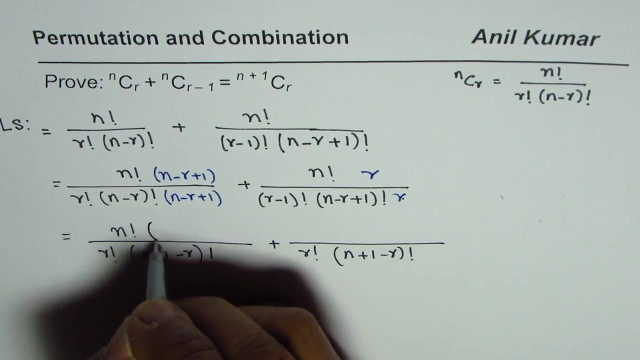 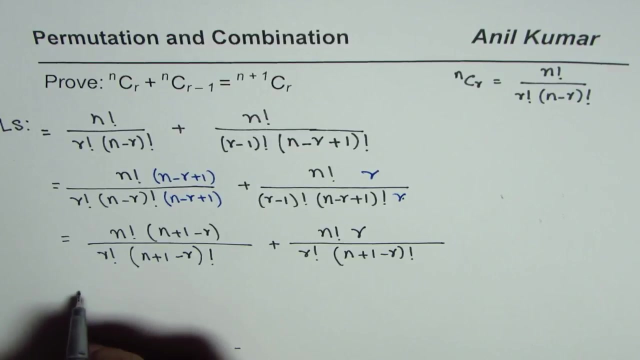 which is r. So this times r minus 1 factorial is same as r factorial, and this one could be rearranged and written as n plus 1 minus r factorial, And the numerators for us are n factorial times, n plus 1 minus r and this is n factorial times r. Now, since the denominators are same, 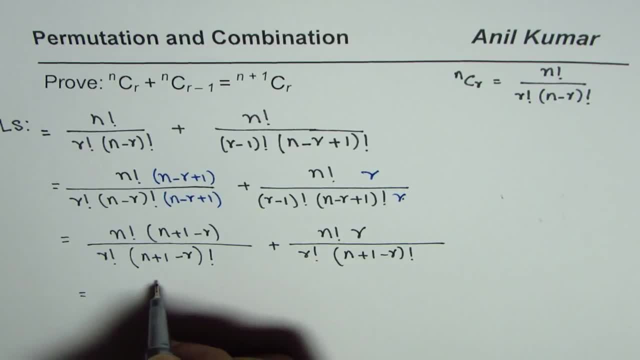 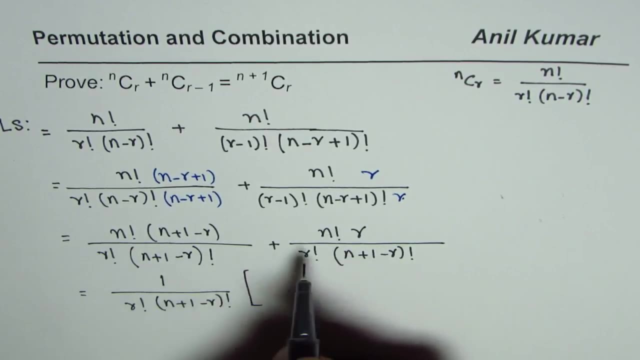 we can take them as common. So what we have to do is we have to write the terms in the denominator. So what we have here is 1 over r factorial times n plus 1 minus r factorial, and in the numerator let us add them. I should actually take n factorial also common right. So we 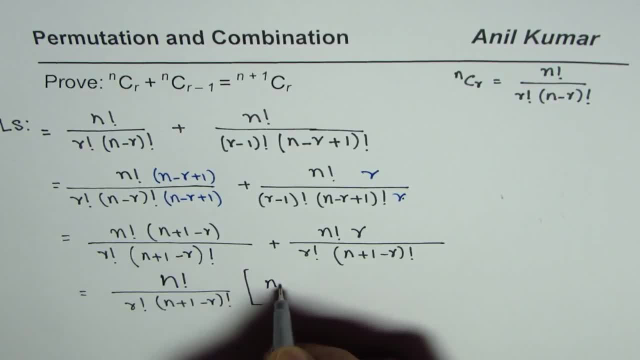 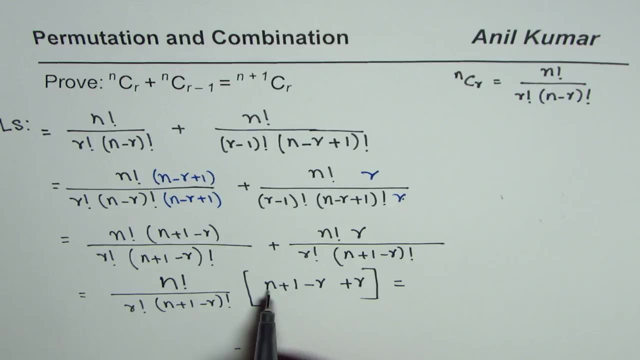 have n factorial also common. We have the terms n plus 1 minus r, and here we have plus r. that is equal to what? Now, clearly, minus r plus r is 0. So we are left with n plus 1 here, right, So n plus. 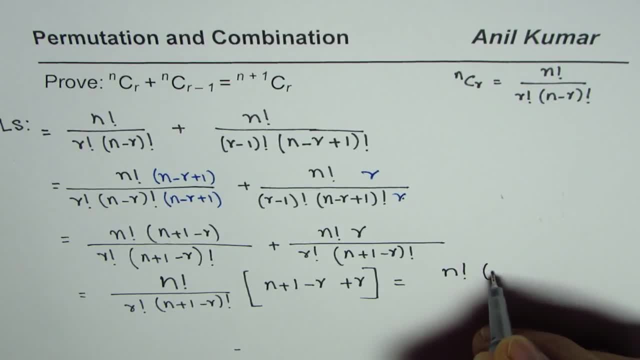 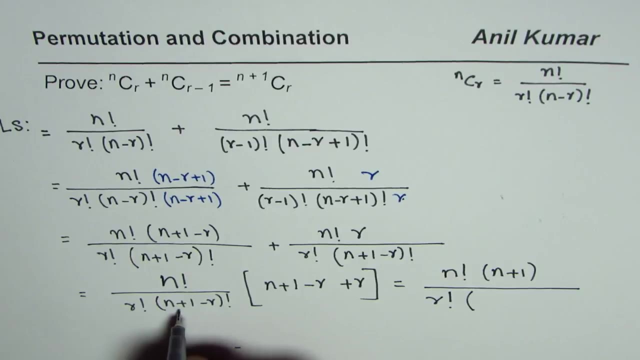 So this becomes n factorial times n plus 1, and the denominator for us is r factorial times n plus 1.. So this becomes n factorial times n plus 1.. And the denominator for us is r factorial times n plus 1, minus r factorial times n plus 1.. 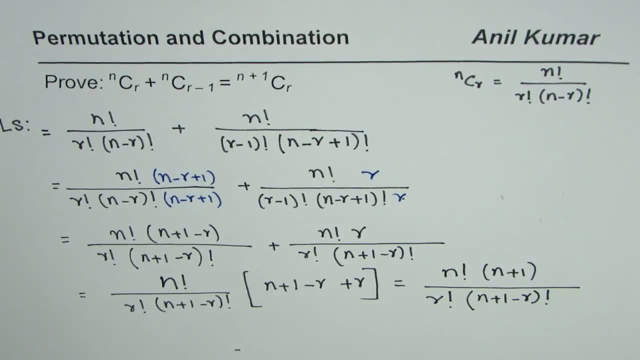 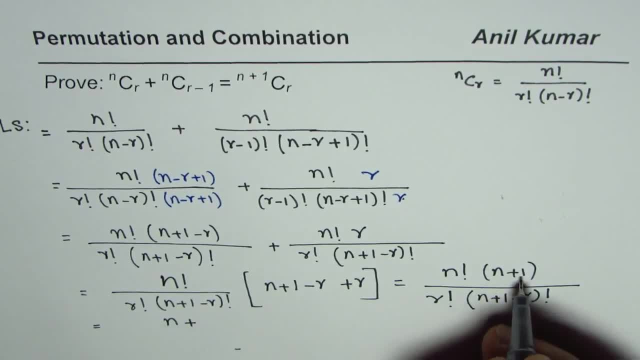 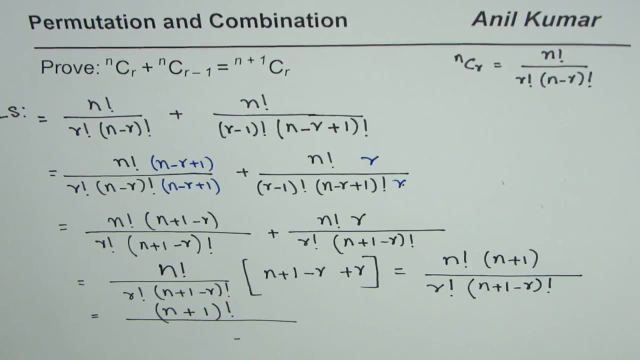 Let me rewrite this as n plus 1 factorial divided by r factorial times n plus 1 minus r factorial. So in the term of the binomial coefficient we could write this as n plus 1 C R, correct? So that is how we can say that n C R plus n C R minus 1 is equal to n plus 1 C R. So